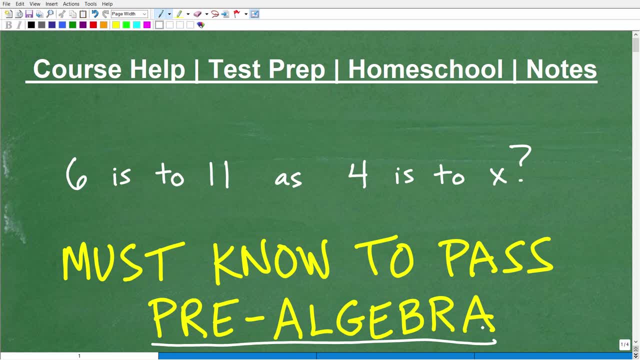 So let's go ahead and review the problem and see if you can actually get the answer. And here it is. So it's 6 is to 11, as 4 is to x. okay, as 4 is to what number. Now I'm not going to really comment any more about this problem right now because I want to give you an opportunity to think about it and solve it. So go ahead and put your answer into the comment section, if you know how to solve this, And also tell me what the description, what type of what's the math topic that we're studying here? 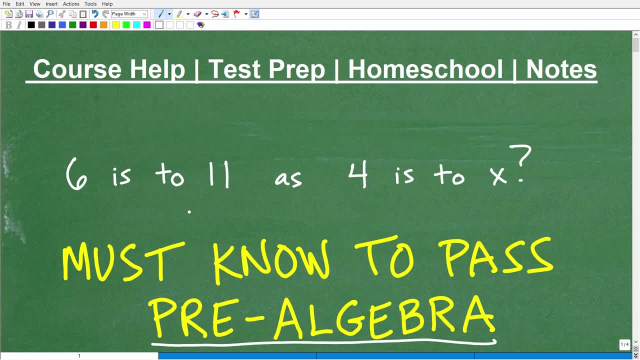 Okay, so if you know what that is, then that's you know really, really good. But again, this is kind of like you know stuff that you have to do or really kind of have to know at the pre-algebra level. 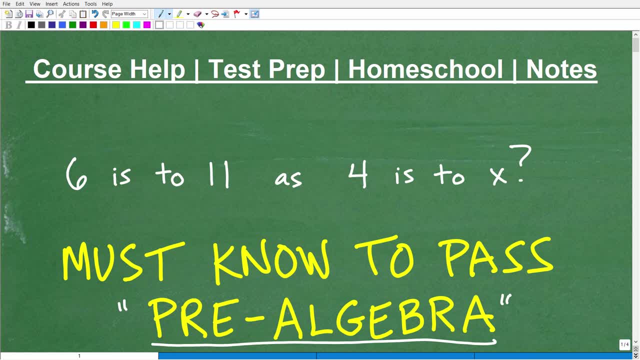 And you're going to have a tough time passing pre-algebra if you can't do a problem like this. So we're going to get into this. It's not that difficult. But I want to talk about all of this in just one second. But first let me quickly introduce myself. My name is John. I'm the founder of Tablet Class Math. I'm also a middle and high school math teacher. 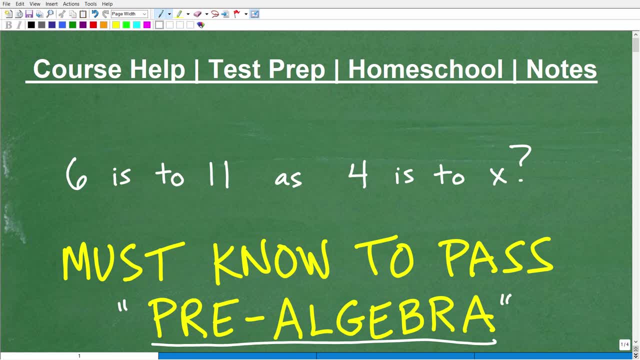 I'm going to leave a link to my master's math help program in the description of this video. but if you are having a difficult time in mathematics, maybe you think you're bad at math. i'm here to tell you that that's not true. okay, as long as you have the desire to learn math, what you need is the right instruction. 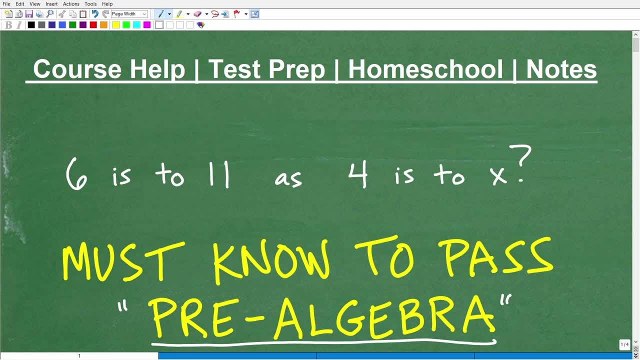 okay. so if you don't feel like you're getting the right instruction or enough instruction, then i've been teaching math for decades and i really teach differently than a lot of teachers. i really try to explain things in kind of like real, super clear, bite-sized pieces. 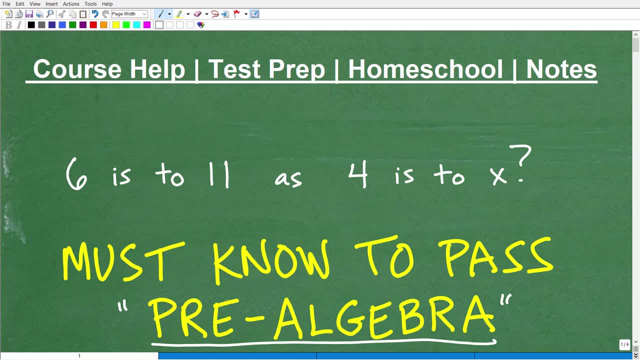 so anyone and everyone can understand this stuff, and anyone can. as long as you're willing to put the work in, i think i have the right instruction for you. so if you're at the middle school, high school or college level in your math courses, i can help you out now if you're preparing for 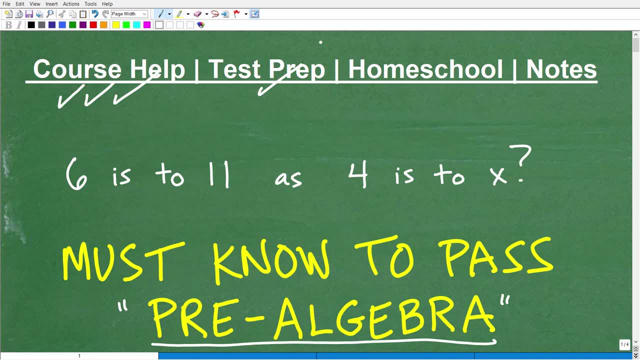 any kind of test that has a math section on it. i'm talking about things like the ged, sat act, gre, gmat, asfab, acuplacer clip exam, maybe a teacher certification exam. i can help you prepare and pass those exams. if you homeschool, you got to check out my homeschool math courses. we were just voted number one for middle and 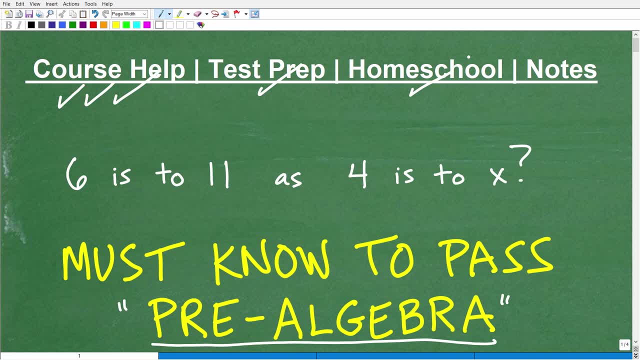 high school math by a major national publication. very, very excited about that, and if you need some math notes, i'm going to leave links to my notes in the description of this video as well. but you're going to have a tough time getting great grades in math if you're. 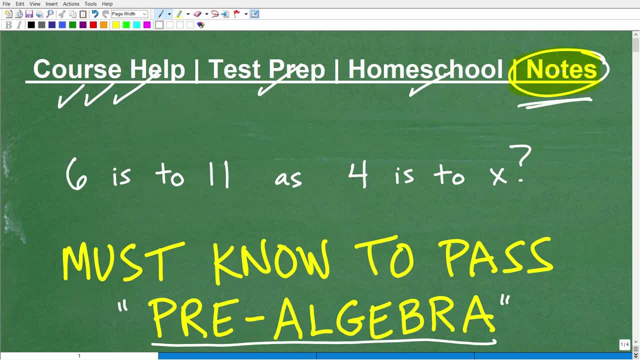 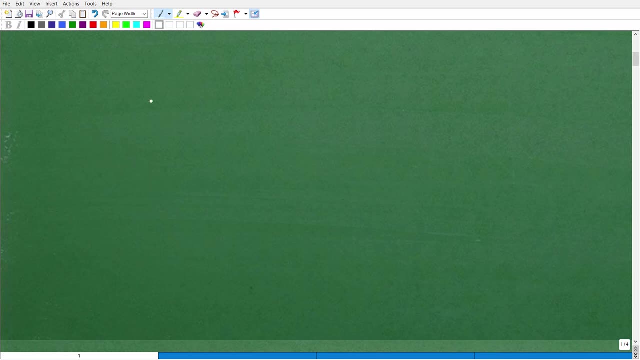 not taking great math notes. so start improving your notes and you'll start seeing everything start to improve like magic. okay, so let's get into this problem. six is two eleven, as four is to x. so what is the topic that we're dealing with, okay? well, let me go ahead and give you. 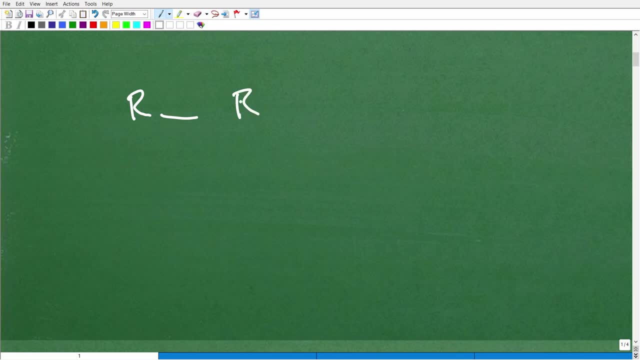 some uh letters here, so it's typically written this way and it's kind of i'm gonna have like fill in the blanks. so, uh, and i'll put some commas in so that we're talking about three words: one starts with an r, another one starts with r and the other one starts with a p. so 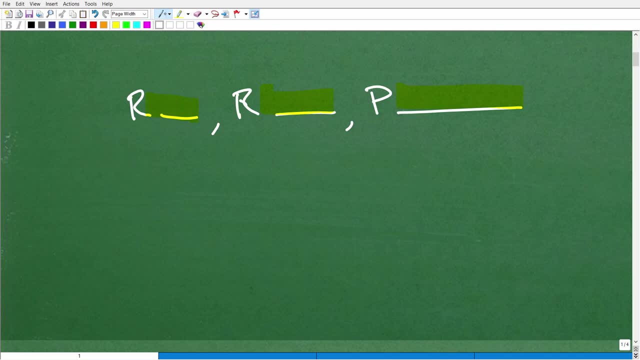 can you guess what those are? okay, put those into the comment section if you know what it is. so what are we talking about? what we're talking about here? we're talking about the word ratios, rates and proportions. okay, so ratio, rates and proportions and this particular problem, um, we're dealing with ratios, so ratios, use the word two. okay, rates, uh, use the word. 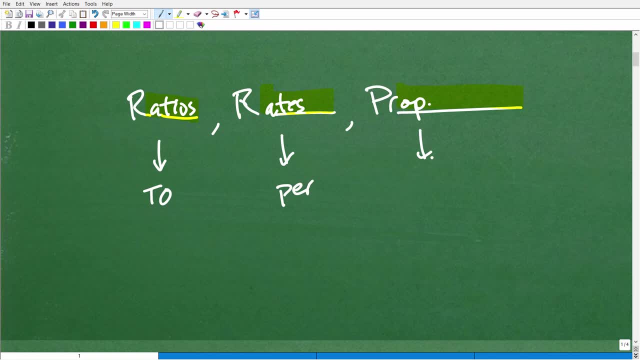 per and a proportion is something called two equal fractions. let me give you an example. this: so two is like the problem that we're dealing with right now. so if i say uh, two, uh, that's, i'm using the word two. how about a different word? three is two, seven, okay, this. 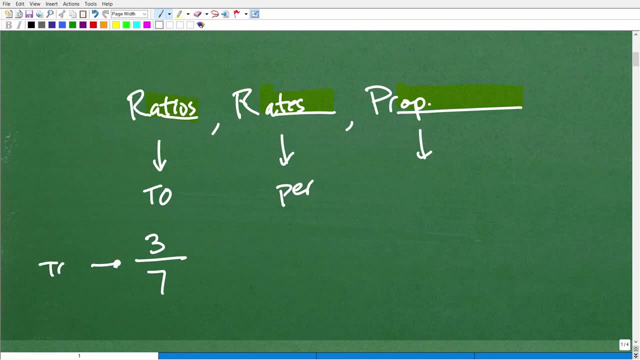 is three, and then this little fraction bar, we use the word two, seven, okay, three is two, seven per would be like, uh, 20 miles okay, per, one gallon okay. so if you notice, here we're talking about different units of measure. that's a rate and i'm just doing a quick, quick, quick. 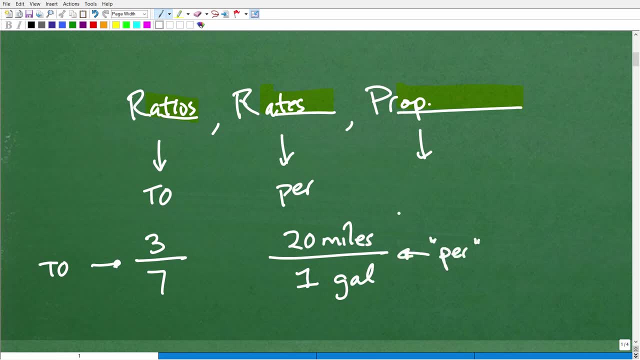 review of how far we would use the word per. that indicates a rate and um uh. you can see that this is a rate because the units of measure are different. we're comparing distance with uh- volume. all right, now, ratios is when we have the same units of measure and uh, i don't. 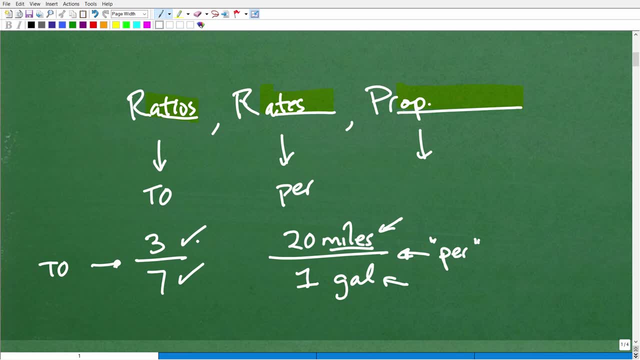 want to go too deep into this because, uh, you know, i'm kind of making uh, this video into a complete overview of all these particular topics. but i have videos on rates, ratio, proportions, additional videos on my youtube channel. of course i can put them in the description box. 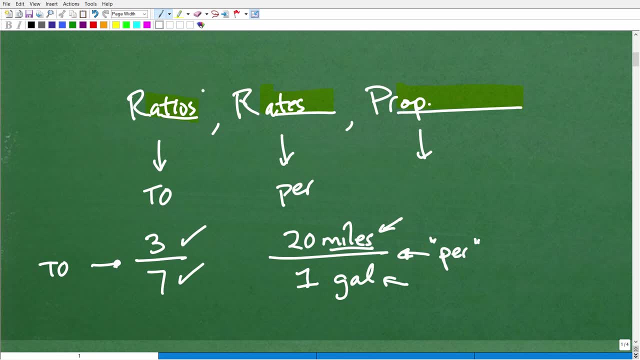 i teach this super thoroughly in any one of my algebra courses. but just as a general uh kind of overview, we were talking about ratios, uh rates, okay, and these are both uh types of fractions. there are fractions with particular type of units of measures, and proportions are two equal fractions. so if i have the fraction one half and i um write another fraction, that's. 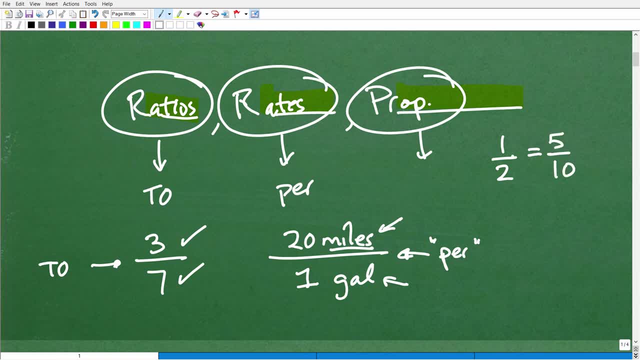 equal to one half, maybe like five over ten. okay, two equal fractions are technically a proportion and the characteristics of a proportion is the cross products are equal, okay, in other words, if i multiply across, if you have two equal fractions, so here one times ten is equal to two times five. okay, so one times ten is ten, two times five is ten, so ten is equal. 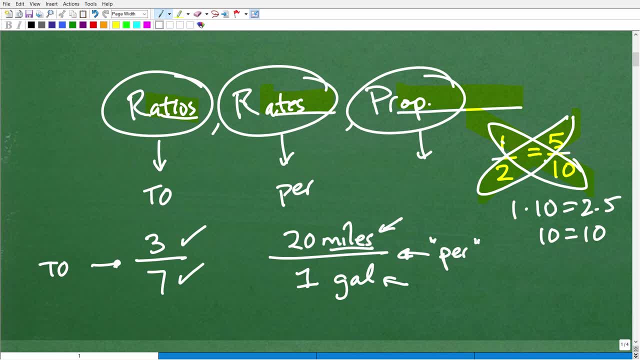 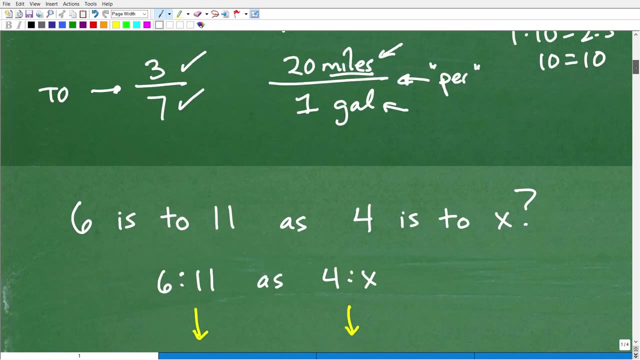 to ten. so when you're dealing with proportions- ie two equal fractions- we know that the cross products are equal. okay, so this is just a quick, quick overview of this particular topic that you study pretty thoroughly at the pre-algebra level and beyond. but uh, now let's go ahead and get into our problem. 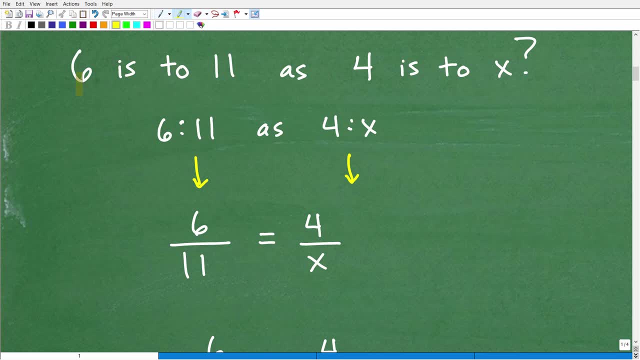 and uh, let's go ahead and read it. so we have six is to eleven, okay, as four is to x or what number? now, we can also write this this way. in other words, you can see this problem written with these, uh, with this colon, like this: okay, so this is another kind of notation for um, the word two, so this six. 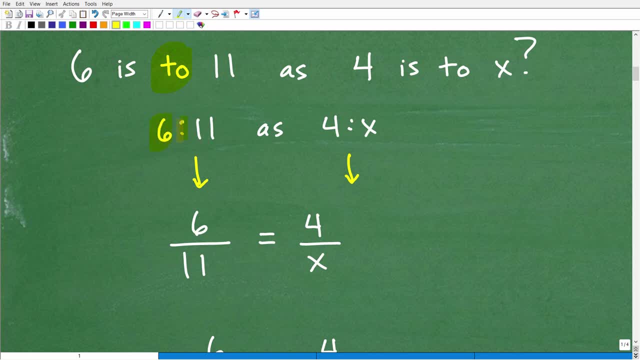 and this uh symbol right there, this colon right there. this means six to six is to eleven, as four is to x. now, you didn't have to write this this way, i just put this in just uh as an aside, because you need to understand this notation, right there? okay, so six uh is to eleven as four is to x. so the key. 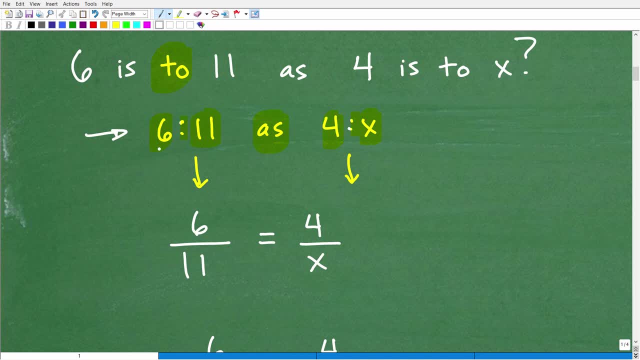 here is to write: uh, these as fractions. so the first number is going to be our numerator and our second number is going to be our denominator. all right, so this is going to be the numerator, this is going to be the denominator, so let's go ahead and do this. six is to eleven, so six. the fraction bar means the word two. okay, so six. 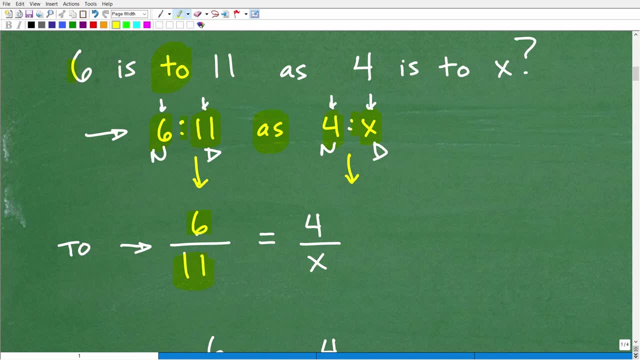 is to eleven. all right, so i'm writing this here as a fraction, as okay, that means equal. okay, six is to eleven, as four is to x. okay, so here, what do i? what am i setting up? well, i'm setting up two equal fractions. i have one fraction and i'm saying it's equal to. 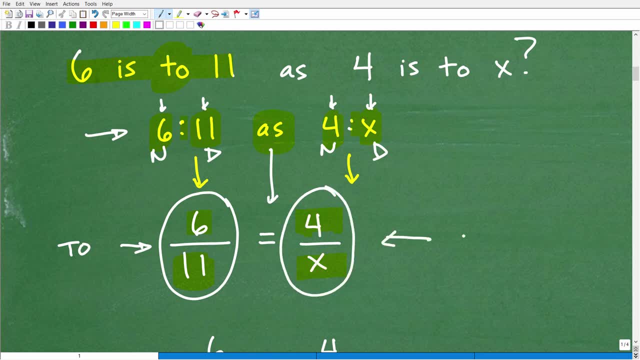 this fraction right there, okay. so this right here is actually a proportion. all right, two equal fractions, and you're like, oh, okay, proportion isn't that? uh, where the cross products are equal, and, yes, you would be absolutely right. okay, so this times this: okay, six times x is going to be equal to eleven. 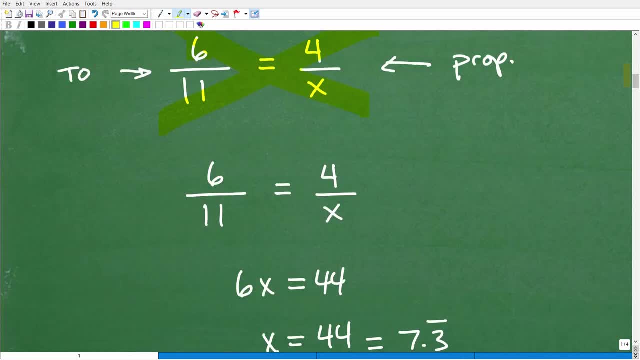 times four, and that's how we're going to be able to solve for x. let's go ahead and do that now. so six times x is, of course, 6x, 11 times 4 is 44, and to solve this basic equation. hopefully you're. 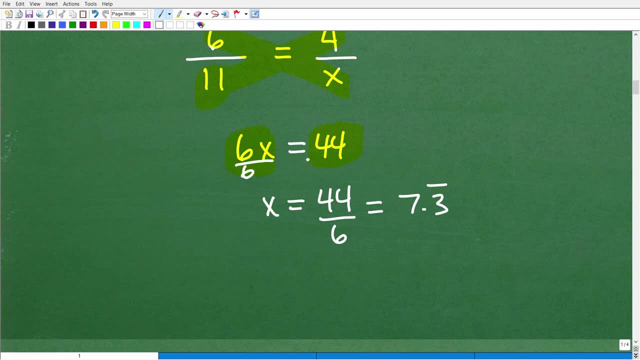 up to speed on your basic algebra equations. all i need to do is divide both sides equation by six, so i'll get: x is equal to 44 divided by 6 and if you want to break out your calculator, you're going to see that that's equal to 7.33333. the threes keep going forever, so the three is: 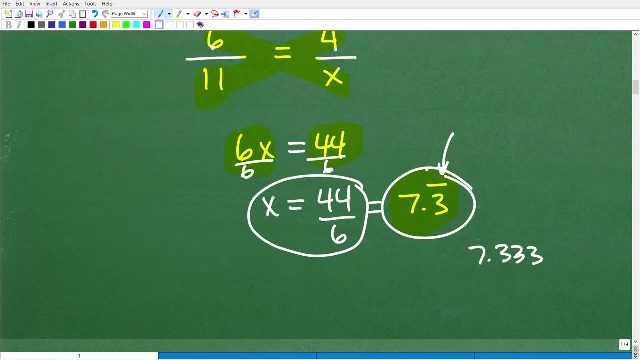 repeating, so you can put a nice little repeating bar over that. but that is the answer, all right. so how did you do? okay, did you get that right? well, if you got that right, then i must go ahead and give you a good old 1982 happy face with the good. yeah, let's put a flat top in. 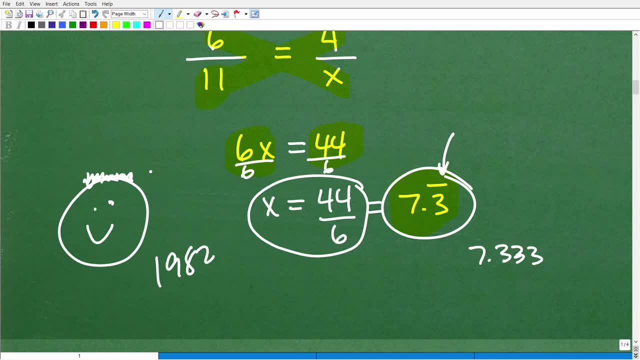 there, uh, these flat tops go back for many, many years. i think they were wearing those flat top haircuts- definitely in the 50s, uh, but in the 80s it was pretty cool too. all right, so let me give you an, a plus. that's cool and 100 nice job. okay, i don't see the flat top haircut around anymore. it's uh.